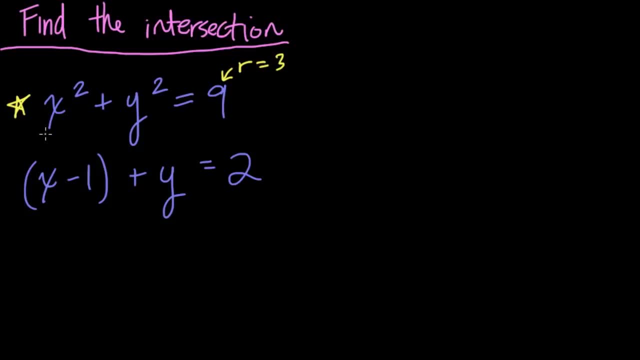 And you might also recognize that this circle will be centered at the origin. And here you might recognize this as a linear equation, because the exponent on the variables is just 1. When that's the highest exponent, you do have a line or a linear equation. 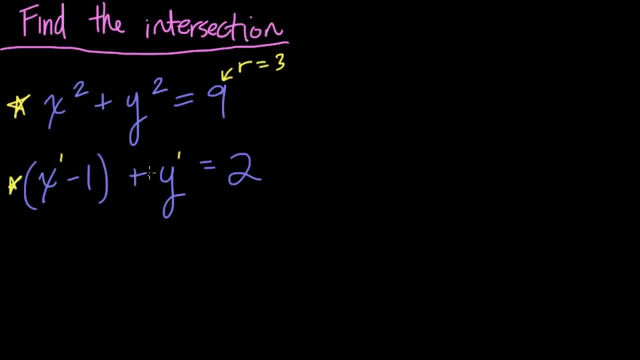 Now to think about what's happening here. right, these two things we hope are meeting at least somewhere, Because what can happen when you have a circle? if you think about this for a moment and a line, how can they meet? 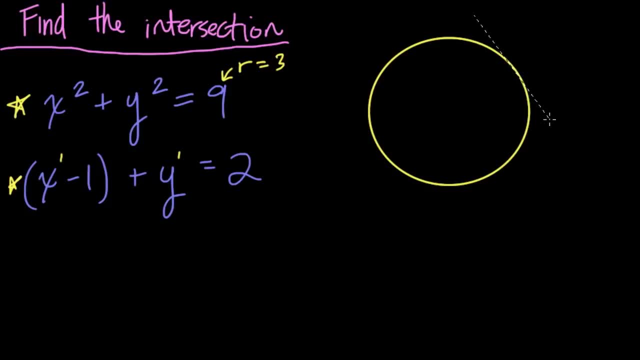 Well, I guess the line and the circle can meet at exactly one point. That's one way it could happen. The line can cross the circle at two points as well, Or the line can never meet the circle, And in the next couple of videos we'll deal with all of these situations. 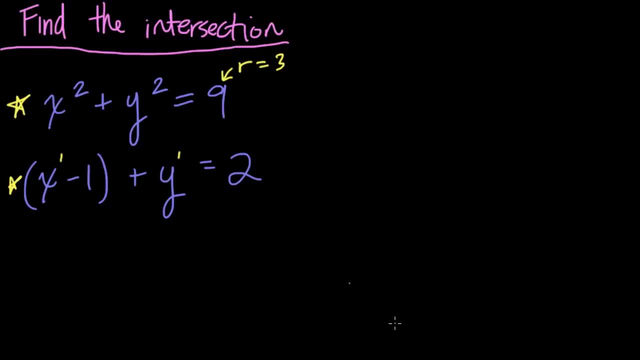 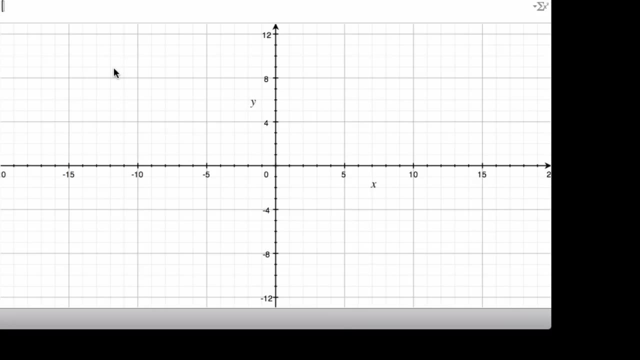 But first let me just quickly graph out these two so we get a sense of what's happening here. You can run lots of programs to graph these things out. I'm just going to use Graffer here that I have on my Mac. So what I'm going to do is set up x squared. 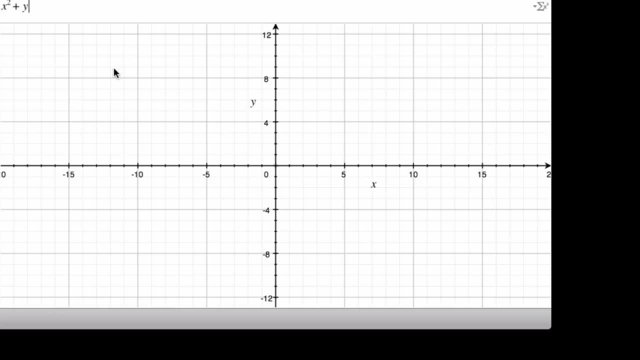 The circle right Plus press down, plus y, squared equals 9.. So we'll see that. And there you see that circle right, Center, at 0,, radius 3. So it's going 3 in every direction. 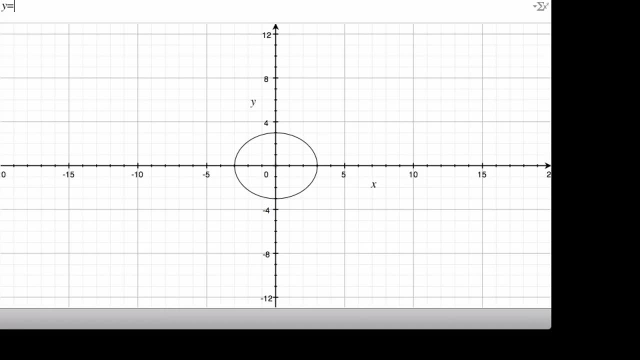 We're going to add another equation. Now let's add in our line: So we have x minus 1, right Plus y equals 2.. And there you can see it: The line is crossing the circle twice. So here we can expect to find right. 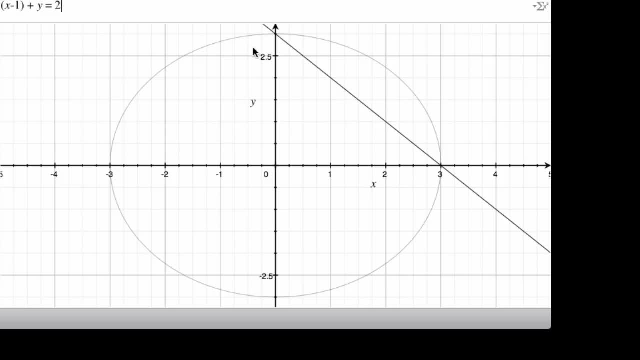 Let's just zoom in for a moment. We can expect to find two solutions And we'll find these two points. You can get a sense of what they are already right. It looks like this point is 3, 0.. And this point up here is also 0, 3.. 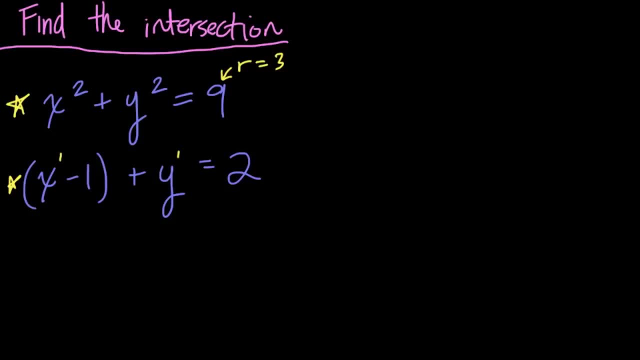 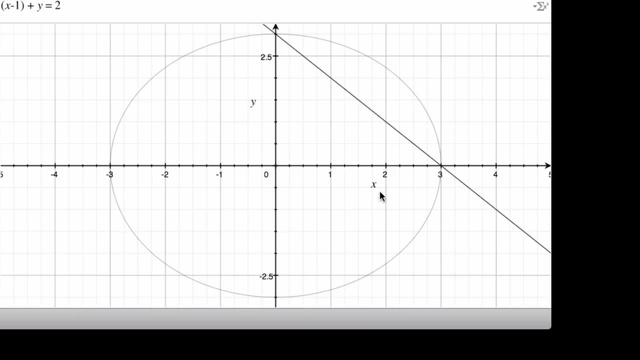 But let's just see how to solve this algebraically. So what do we do? Well, if they're meeting at some point here and here, that means that at these two values- right, These two occurrences, these two equations have the same x and y values. 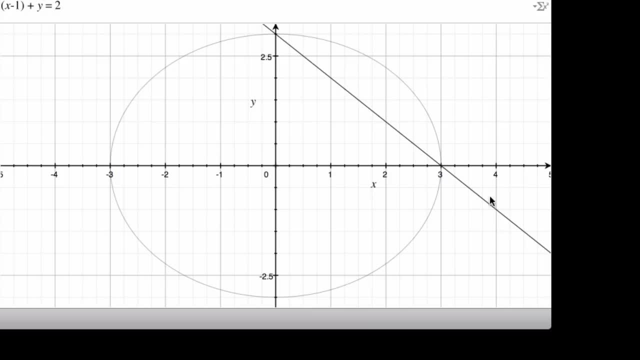 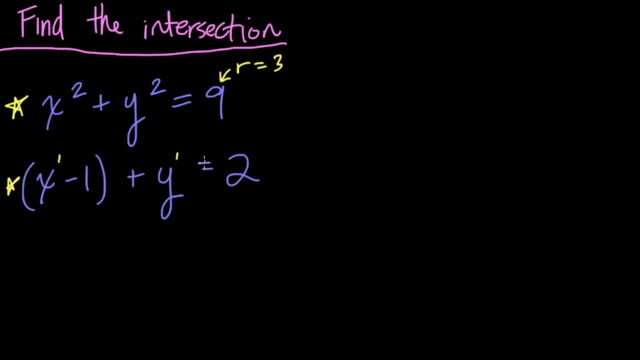 which means they're equal at these two points. They're not equal anywhere else, but they are equal twice To find when these two equations meet and when they're equal. what I'm going to think about is how can I rewrite this second equation so it says something like x equals or y equals. 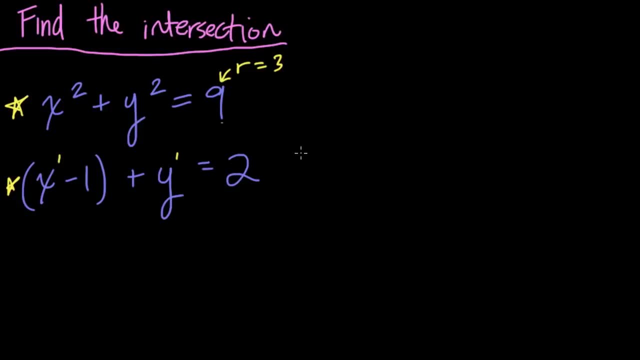 right, the other variable, And then plug it into the first equation. Let me show you what I mean, So I'll write up here different tool. So we have x minus 1, right plus y equals 2.. 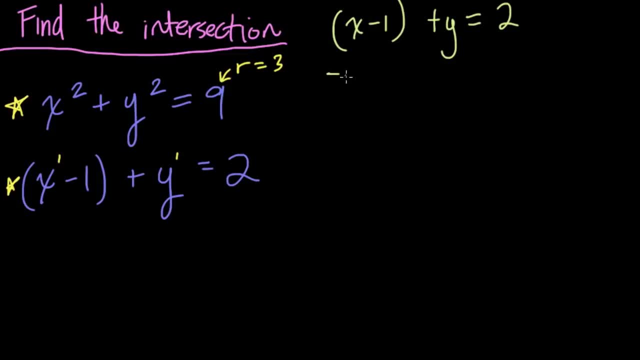 Well, for me it just seems easier to subtract x minus 1 from both sides, because then what will happen? Well, let's just see, right, We do this, This cancels out, and we get y equals 2 minus x plus 1, right. 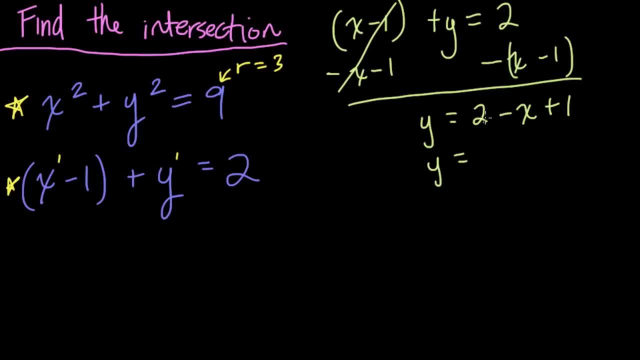 because we're subtracting a negative 1.. And then y equals: well, we have 2.. So we get y equals 2 minus x plus 1, right, because we're subtracting a negative 1.. So we get y equals 2 plus 1, which is 3.. 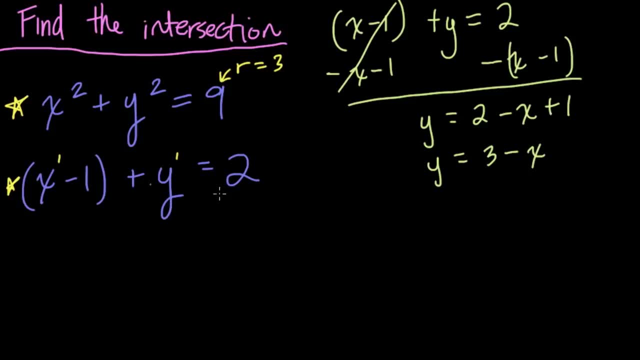 And then we have y equals 3 minus x. So what does this mean? Well, I can now plug this in to my first equation. My first equation says: x squared plus y squared equals 9.. But we know that y is equal to 3 minus x in this second equation. 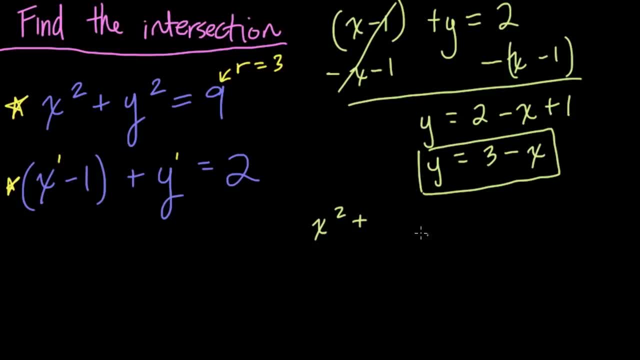 So we can plug that in right, because we're assuming at some point these two things are equal. So here, instead of writing y, I'll write 3 minus x squared, and that's going to equal 9.. Now, this is nice, even though you might feel confused about this. 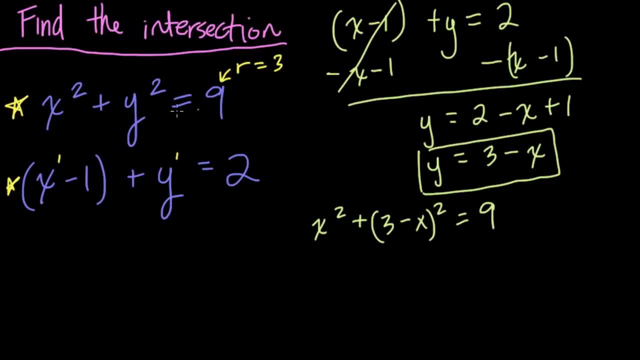 because what's happening here is, instead of having two variables in one equation, we have now one variable x for one equation, And if I expand this, I get x squared plus right. this is 3 minus x times 3 minus x, and that equals 9.. 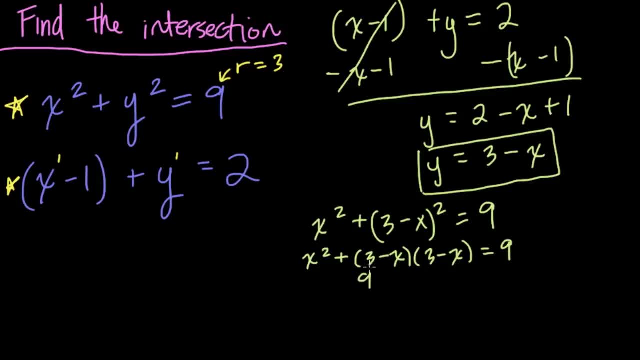 You see the distributive property here We have 3 times 3,, which is 9.. 3 times minus x. Minus x, which is minus 3x, minus x times 3,, which is another minus 3x, and then minus x times minus x. 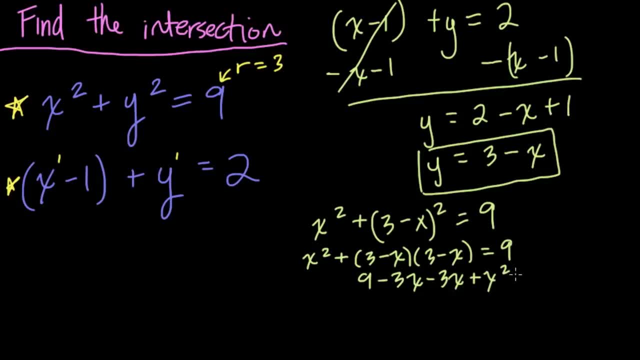 which is plus x squared, and that equals 9.. So we have x squared right, plus 9, minus 3x, minus 3x plus x squared. So if I subtract 9 from both sides and simplify, what's going to happen? 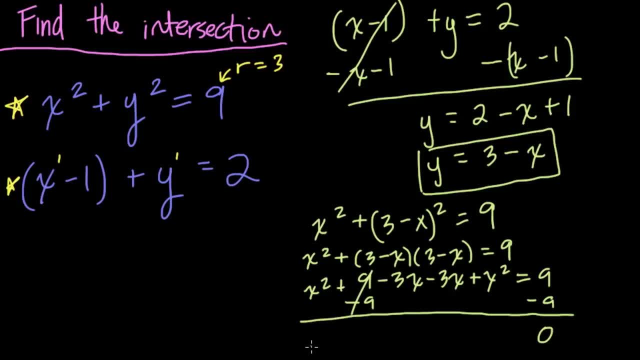 Well, 9 minus 9 is 0.. Over here, these 9s cancel out as well. Let's see. So I have minus 3x, minus 3x, that's minus 6x, and 2x squared, which is just 2x squared. 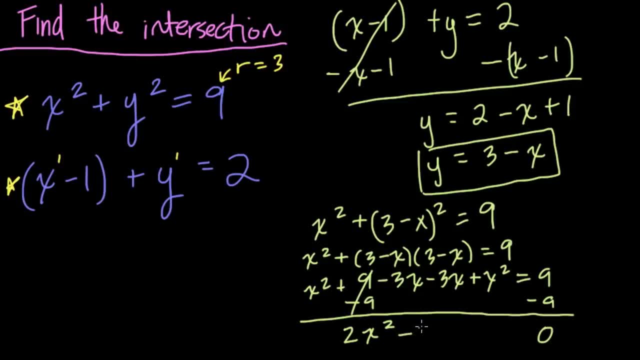 So now we have this equation: 2x squared minus 6x equals 0.. And all we have to do is solve for x. So if I factor out 2x here, I get 2x times right. 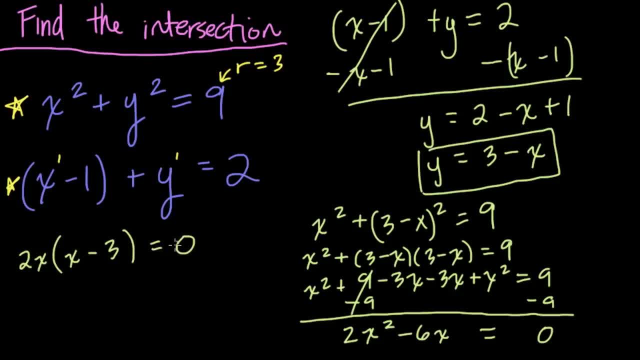 x minus 3 equals 0. So we have two scenarios. now We recognize this. If I multiply this term by this term to get 0, either one of three things will happen. 2x will be equal to 0, right to get a product. 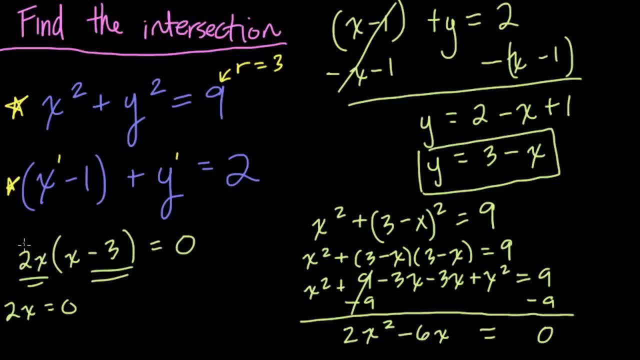 we're multiplying these two of 0. If the first number is 0, then your product is 0. If we solve for x there, we divide both sides by 2, and x equals 0. The other thing that could happen is x minus 3 could be equal. 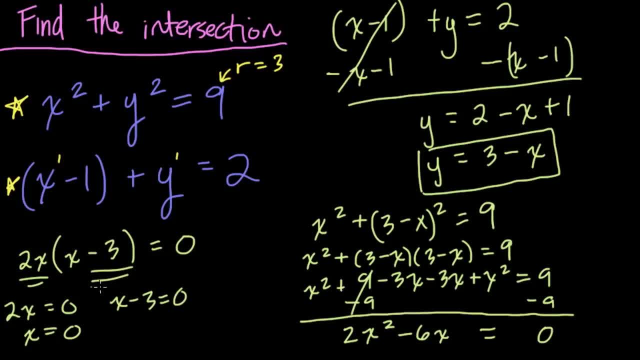 to 0,. right, because if this was equal to 0, x minus 3, that time would be 0. So x times anything would give you 0.. If we solve for x here, we add 3 to both sides and x equals 3.. 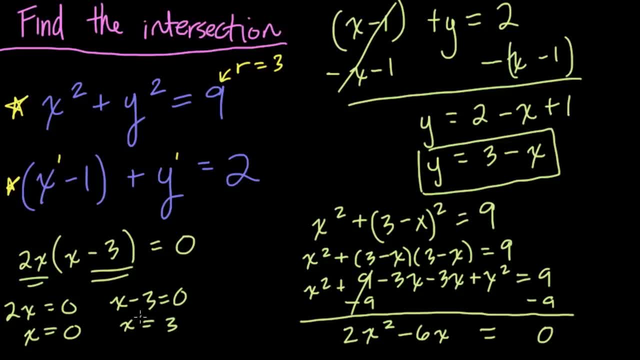 So now either one of these two situations will happen or they're both equal to 0.. We already saw in our picture that both points do work, but if you had to test it out to figure out what which one of these work, you can just plug them in. 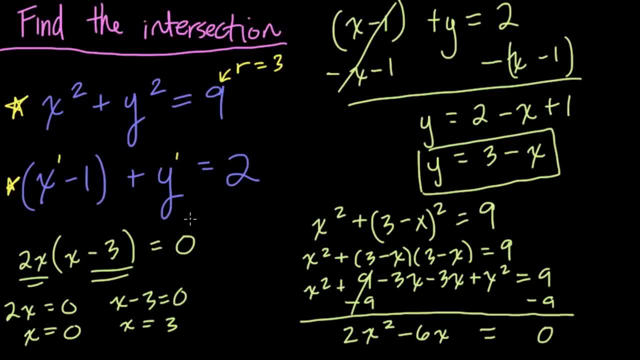 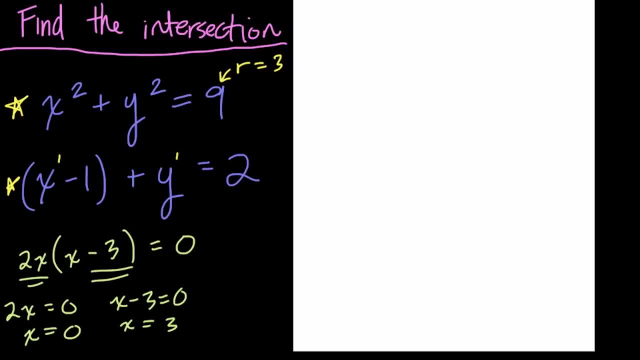 And in fact, we should plug them in because we need to know our y values. We're attempting to find points here, So let me just clear this off, Okay, and fill that in: oops, oops, okay. 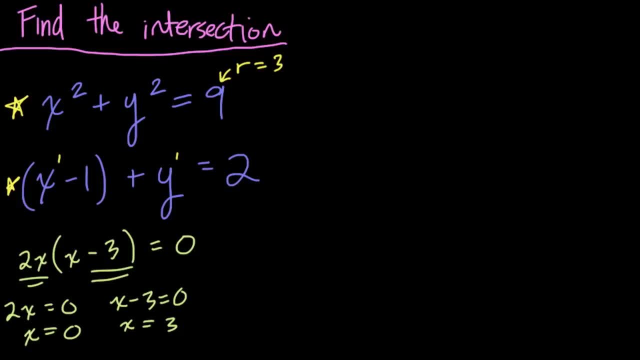 So now, what do we do? Well, we, we. you're assuming we don't know these points here, but we're saying: well, perhaps x is equal to 0. If that's the case, we can plug it now into either equation.